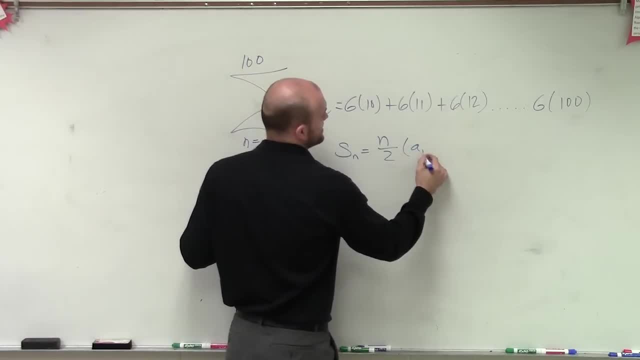 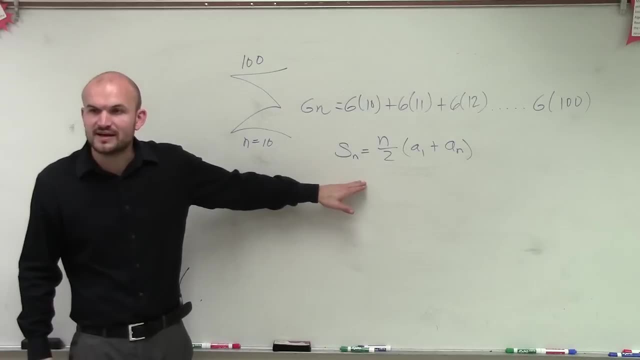 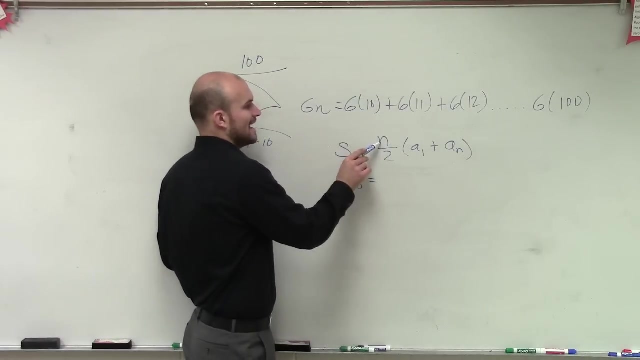 arithmetic sequence is going to be n divided by 2 times a sub 1 plus a sub n. all right, So what they're asking us to do is to find the sum of this series at 100.. So I say s equals 100 equals n, which is going to be so. now we need to determine. 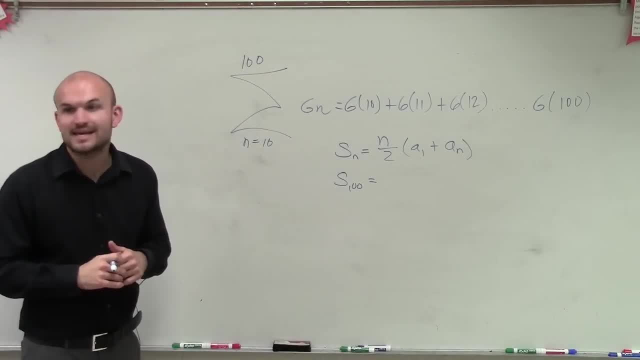 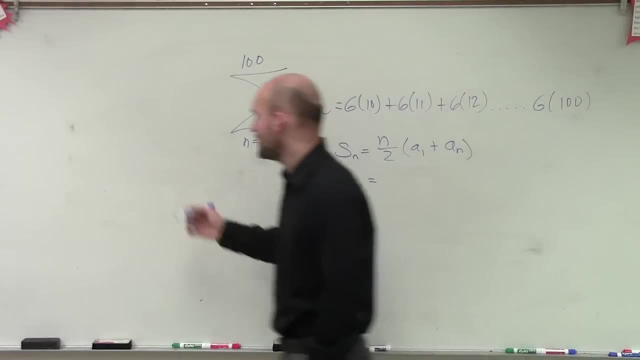 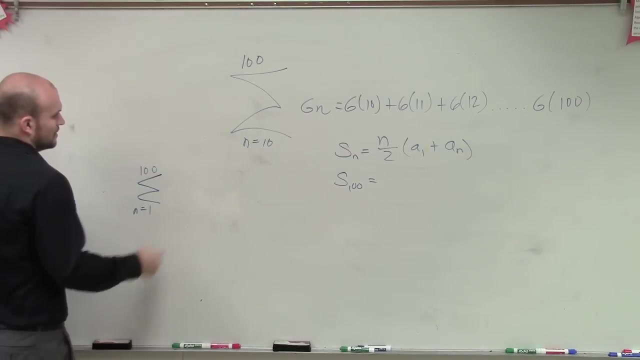 how many values do I have? How many values am I calculating? Okay, Now this is where it gets a little bit confusing thinking about it, because if I had a summation here of 101, we would say n, the number of terms that we're going to find. 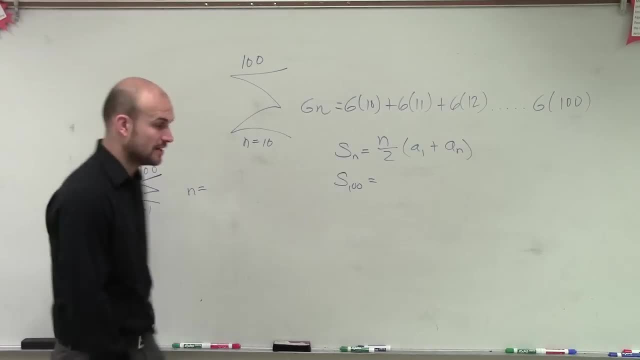 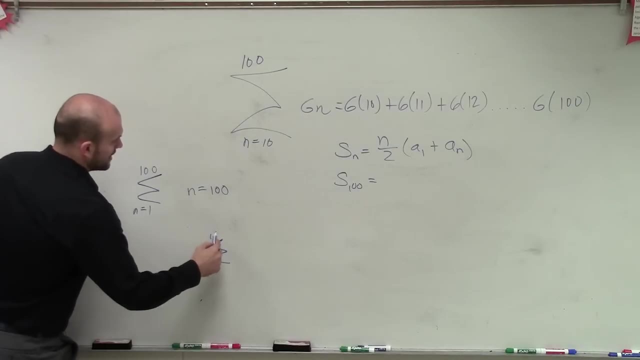 n equals what 100 terms, right, Okay? So now, ladies and gentlemen, if I have a summation and it's going at 100 to 10, okay, well, think about it. How did I get 100?? Did I get 100 by doing 100? 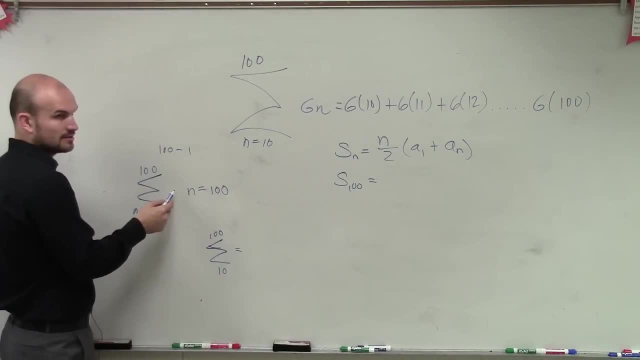 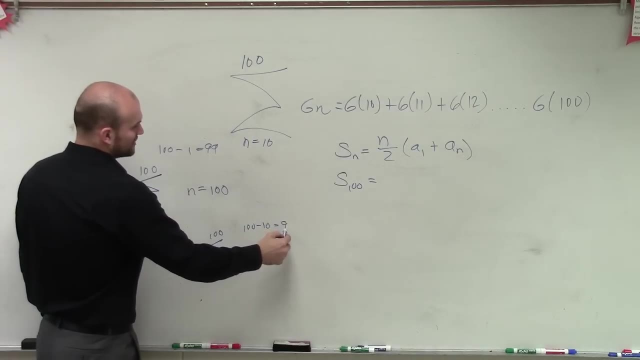 minus 1?? No right, Because 100 minus 1 equals 99. So 10 minus 100 minus 10 would equal 90. But our answer is not 99,. our answer, our n total number, is 100.. So it's not 100 minus 10, but it's actually going. 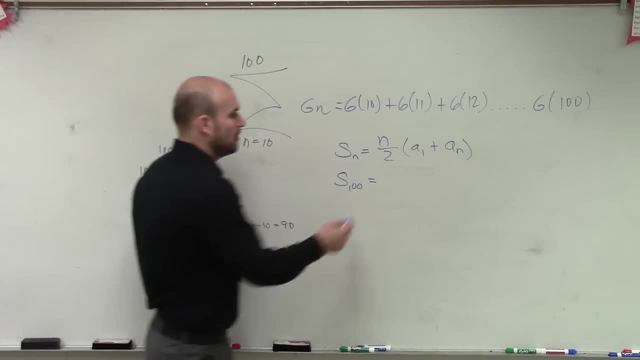 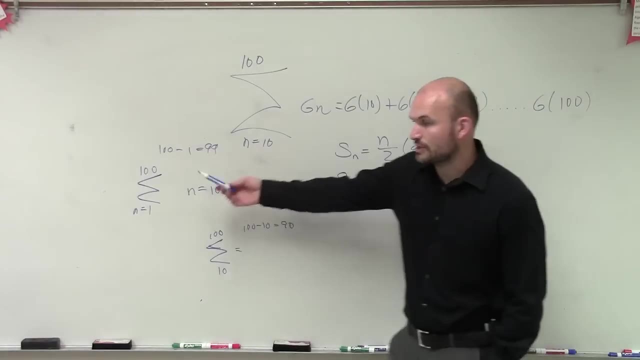 to be an extra term on that, which will be 91. Think about this, Do you understand? if you start at 1 and go to 100, you have 100, you're adding up 100 terms, right? So if you start at 10,? 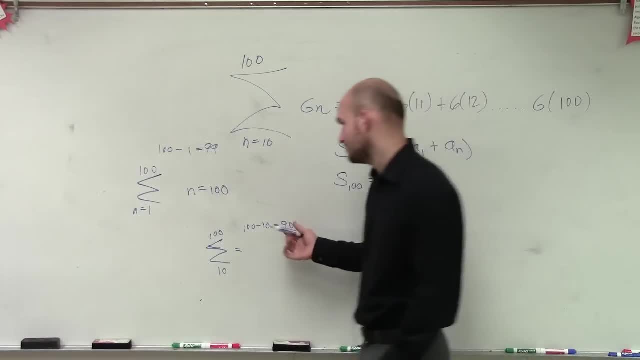 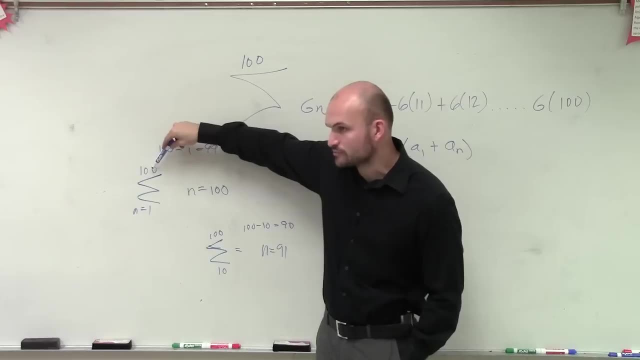 go to 100,. that's not 90. You're just going to be 91. Look it, This isn't 100. You didn't get 100 by doing 100 minus 1.. If you do, if you subtract these like: 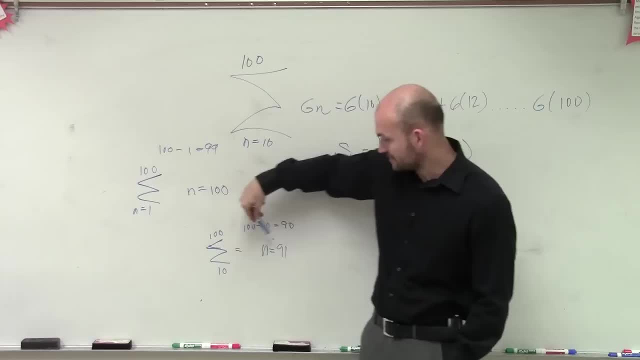 you did here. here you're subtracting to get 90.. 100 minus 10 gives you 90, right? 100 minus 1 is 99.. We said: it's not 99 terms, it's 100 terms. So therefore you're not subtracting them. Well, 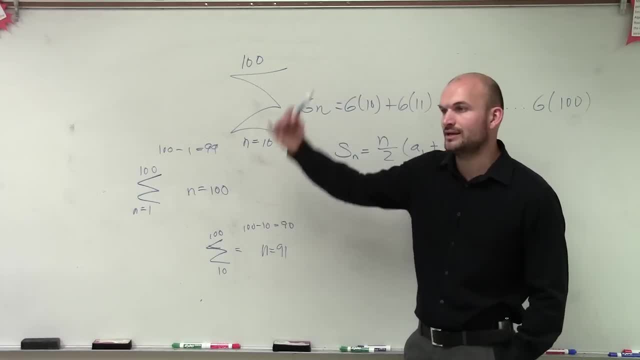 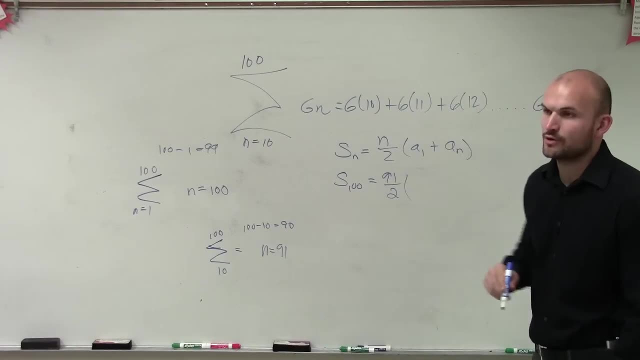 you could subtract them, but you got to make sure you add that extra value, because we're including 10 all the way up to 100.. You're including 10, so it's going to be an extra value, So it'd be 91 over 2.. Now we need to figure out what a sub 1 is. Well, a sub 1 is going to be an extra value.